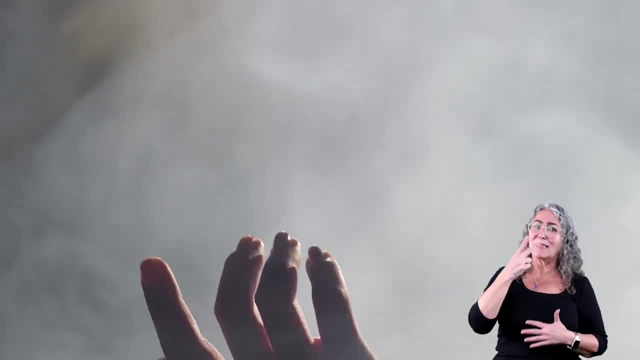 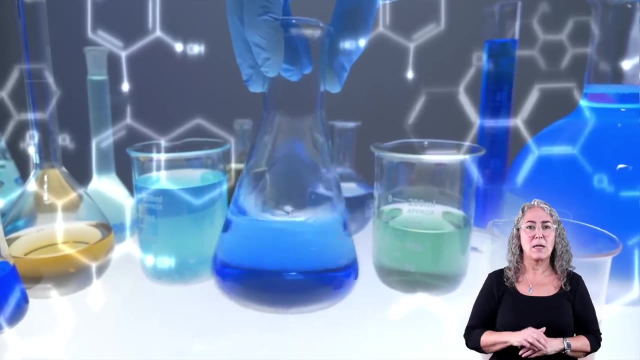 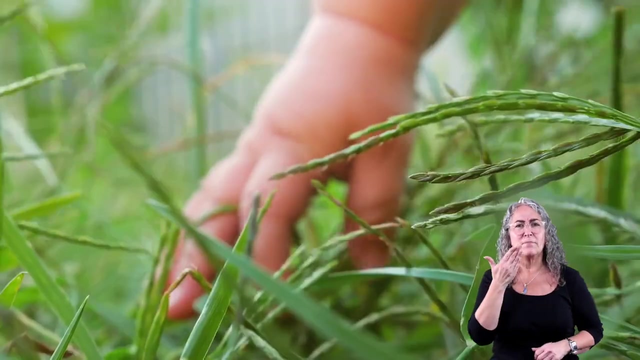 And some stuff that takes up space, like the air you breathe. you can't see or touch at all. We have a word to describe all the stuff in the world that takes up space: Matter. Matter is all-around, Whether you can see it, feel it, touch it, smell it or not. 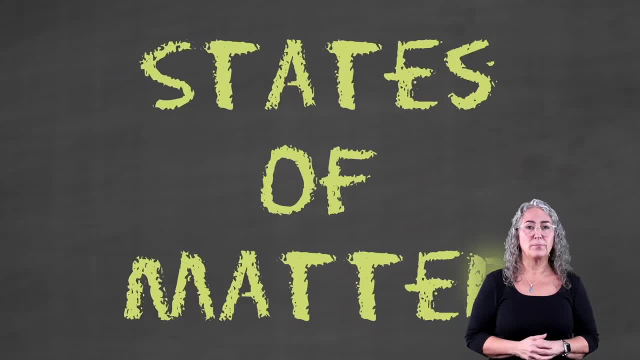 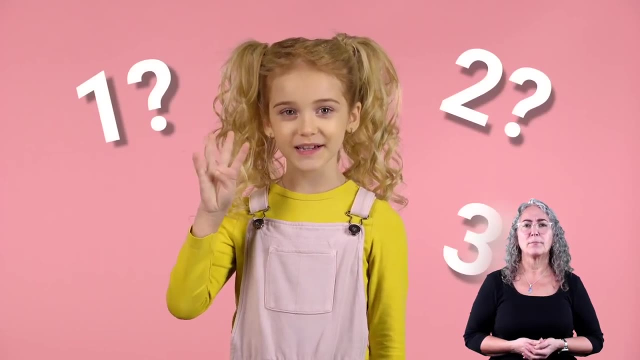 And that's what today's lesson's all about. States of Matter- No, not states that matter. That's a geography lesson for another time. States of Matter- Okay, so think about it. How many different ways can matter exist? Some matter you can hold in your hand like a ball or a book. 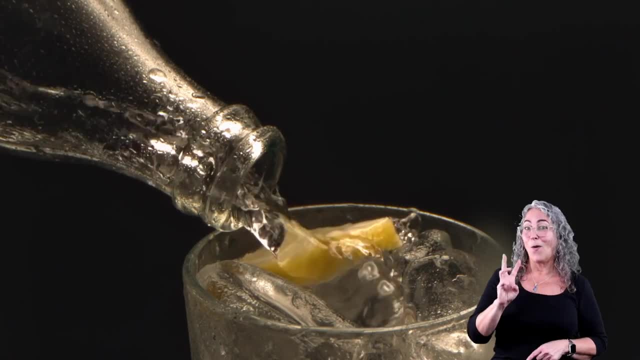 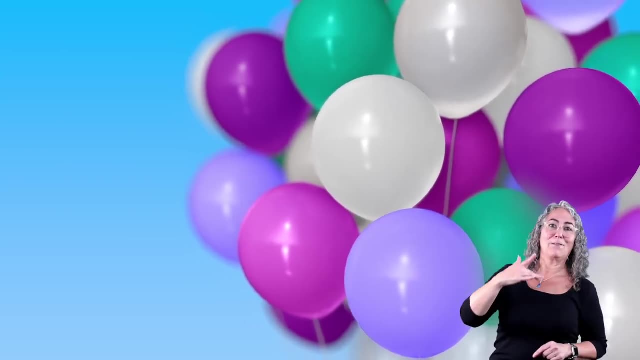 Some matter You can feel but you can't really hold on to, like water or soda, And some matter like air or helium in a balloon, you can't see or feel or touch at all. So there are three different states of matter. 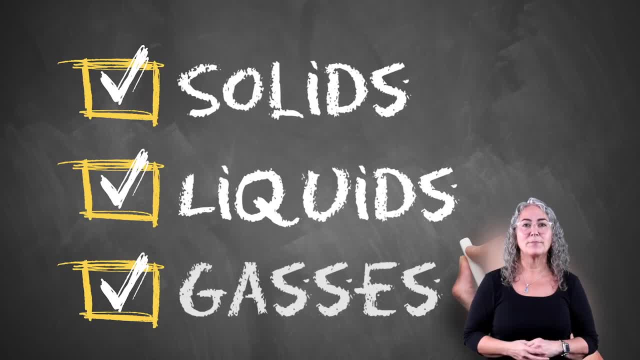 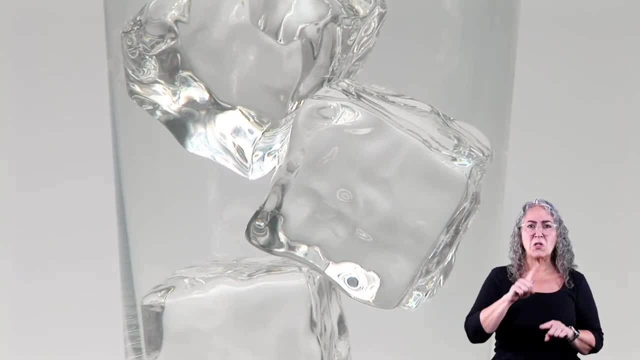 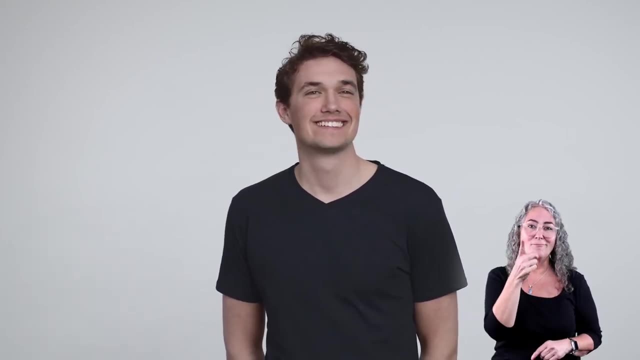 Solids, liquids and gases, And it's pretty easy to tell them apart. I mean, you can't drink a solid right And you can't hold on to a liquid and a gas. They're all around you But you wouldn't even know it because you can't see them. 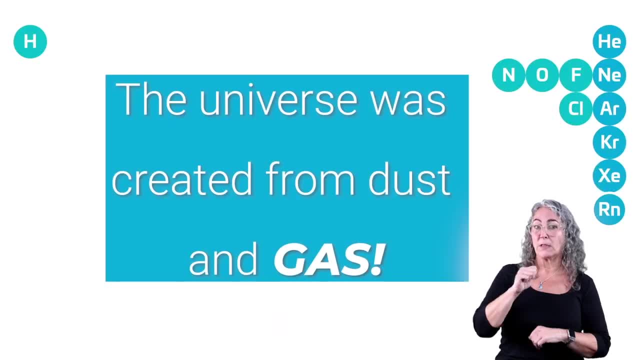 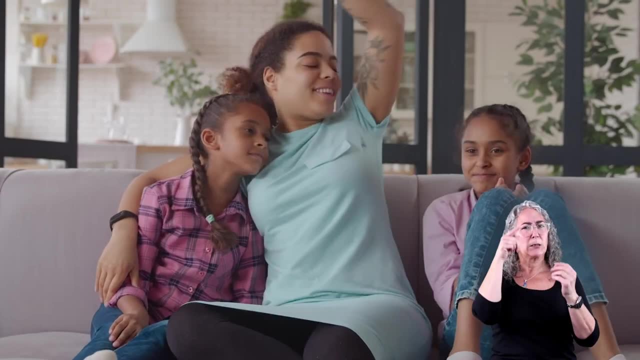 You might be tempted to think that gases aren't as important as solids or liquids, But without gases, none of us would even exist. Do me a solid and think about the chair or couch you're sitting on right now. What's it like? 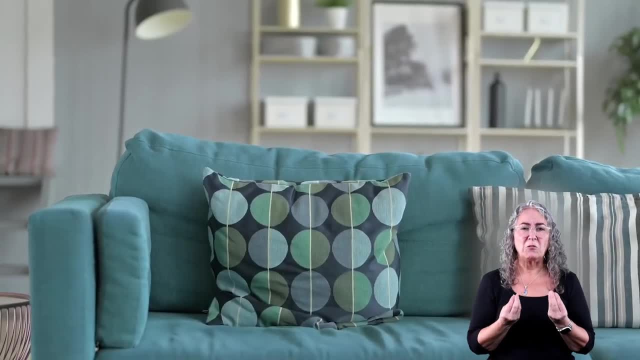 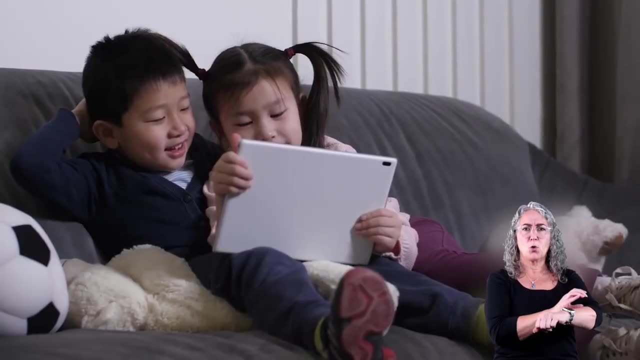 Does it have a definite shape? Is it soft, hard? a little of both. Can you pick it up? Does it make a sound if you tap on it? What about the computer Or device you're watching this video on, Or the bread you ate- last time you had a sandwich. 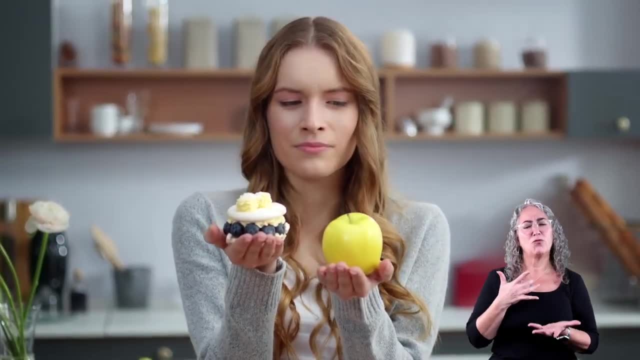 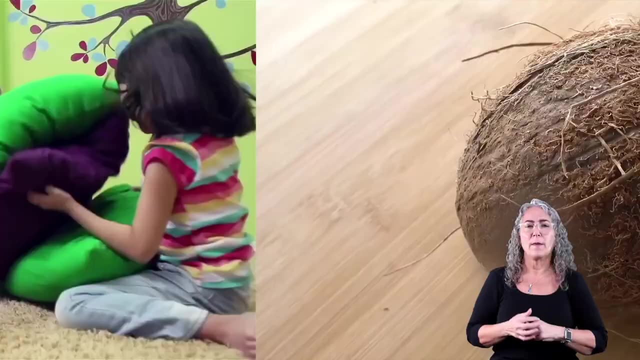 Solids are things you can pick up, hold and feel. the shape of Solids always have a shape. They can be hard, smooth, rough or soft. They come in all different sizes, from as small as a marble to as big as a mountain. 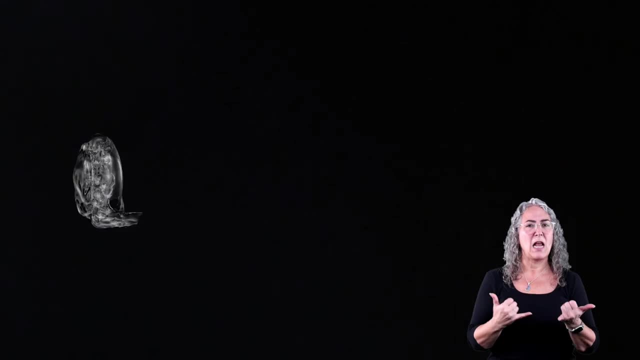 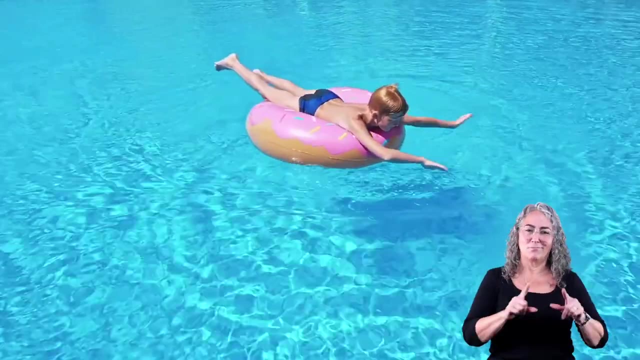 And you can hold them in your hands if they'll fit. Now let's talk about liquids. The most common liquid is water, But there are a lot of other liquids all around you. Ever had a bad cough and been given cough syrup? 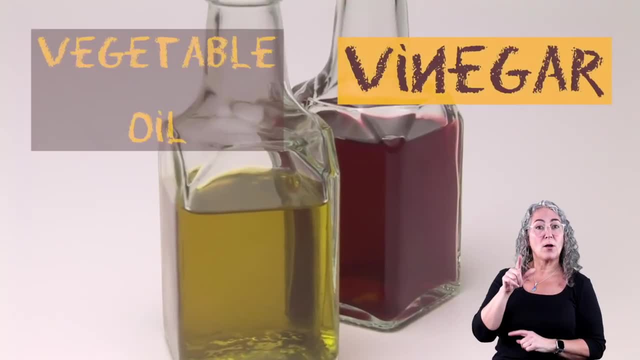 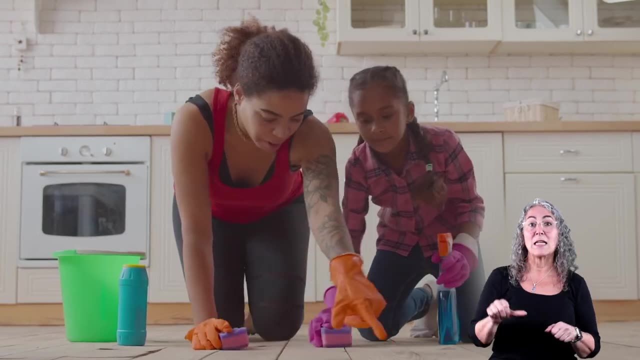 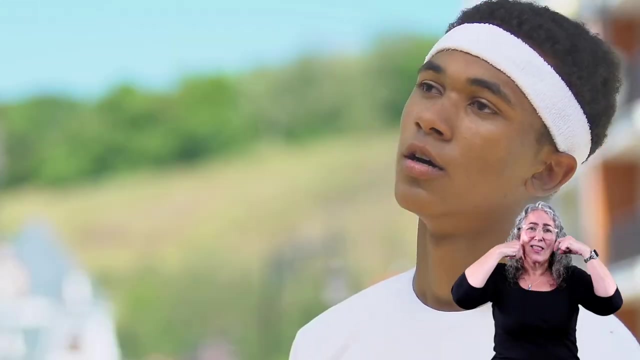 That's a liquid. So is vinegar, vegetable oil, chocolate syrup and the cleaning fluids your parents might use to tidy up the house, The gasoline your parents put in their car or lawnmower- Yep, that's a liquid. So is the sweat that comes out of your body when you run around a lot. 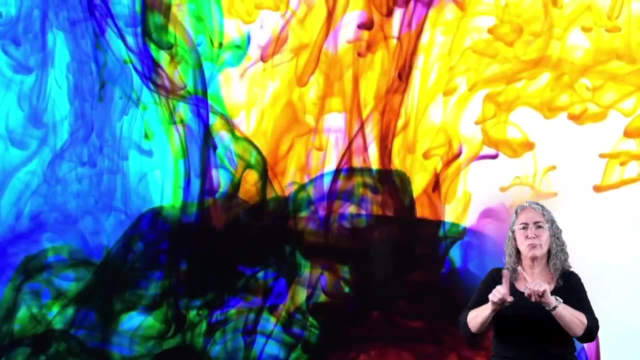 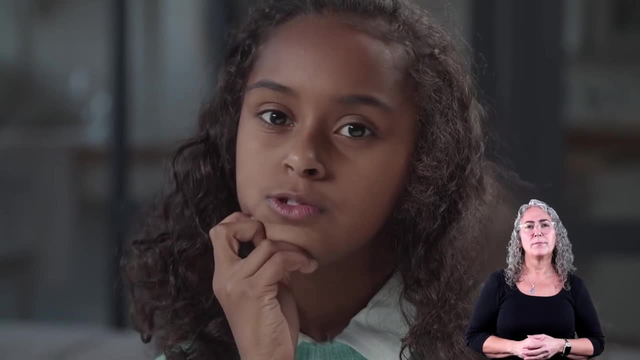 Of course, a lot of the liquids we just mentioned are partially water, But they're still liquids. So can you tell me what all liquids have in common? First, they will always fill the bottom of a container if you pour them in. 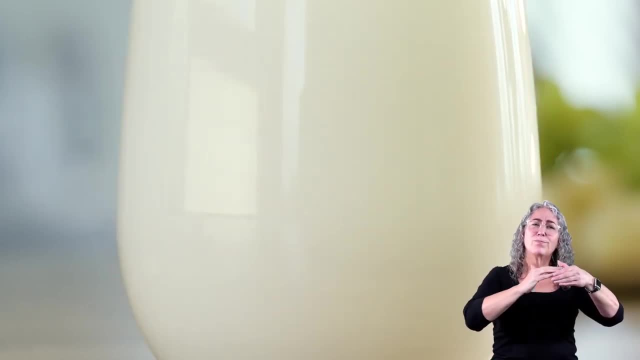 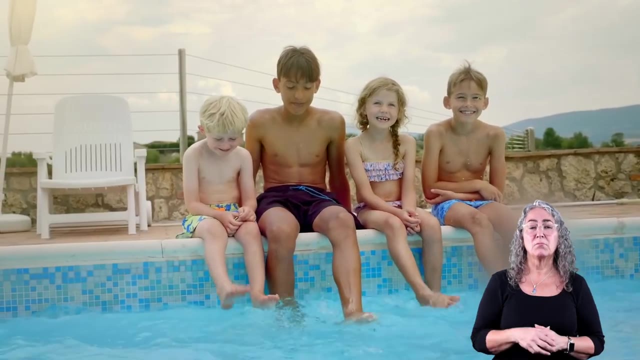 And they'll take the shape of that container as you continue to pour. They usually have a smooth surface, They can be really hot or cold or somewhere in between, And they don't have a specific size. A liquid like water can fill an entire ocean. 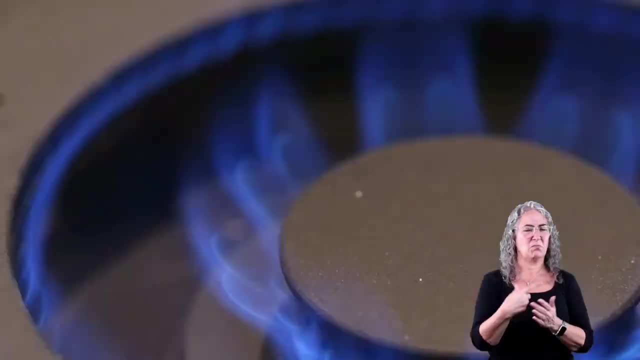 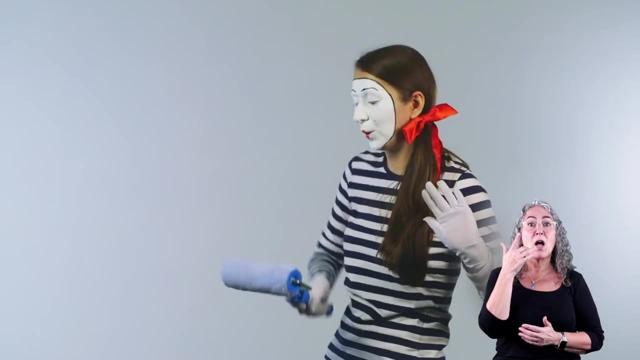 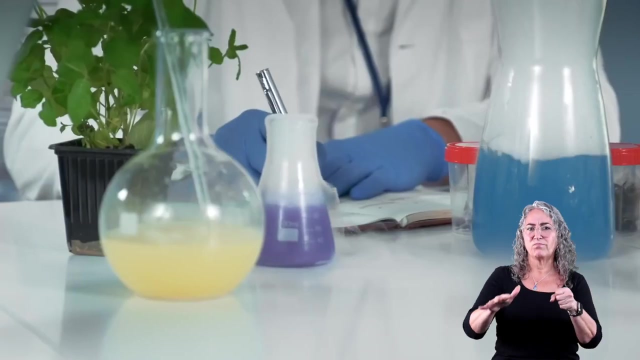 Or the smallest crack in the sidewalk. Okay, now let's talk about gases. Gases are some of the most interesting of all types of matter, Because they're all around you, but you can't see them. A gas is invisible, has no shape or size, can fill any size container and has no surface, and moves around easily. 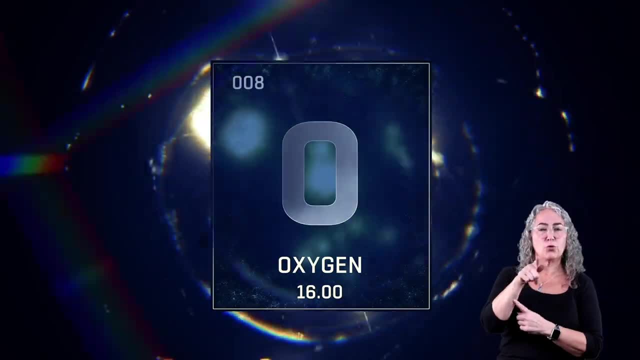 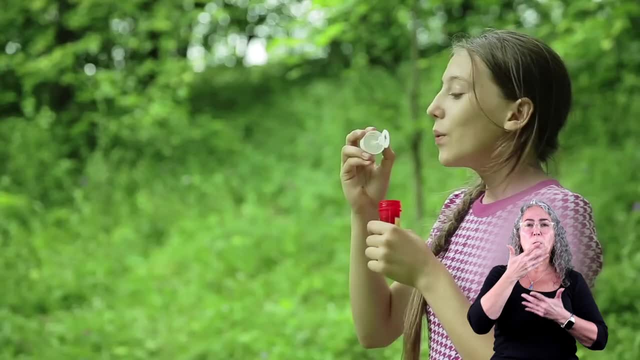 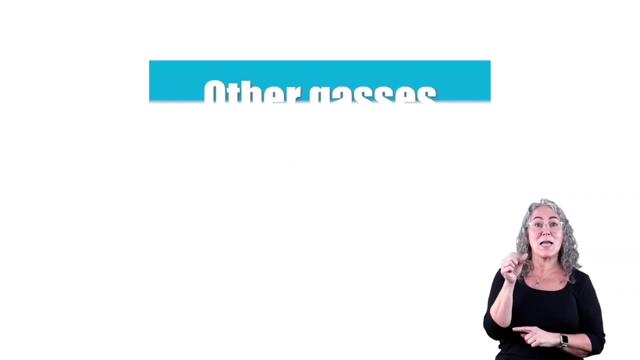 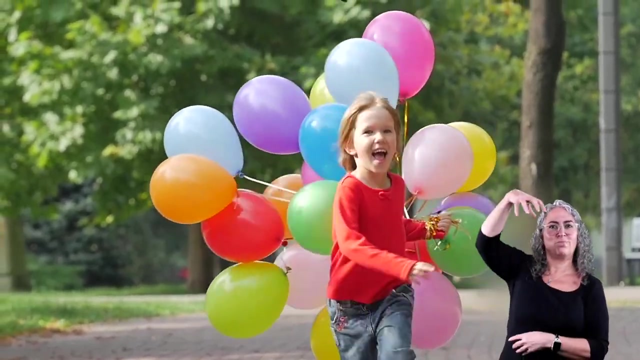 Not to mention CO2, or carbon dioxide, which is a gas that you breathe out. Carbon dioxide gas gets absorbed by the trees around us. Other gases you might be familiar with are helium and propane. Helium is used to fill balloons And, since it's lighter than air, a helium-filled balloon floats upward. 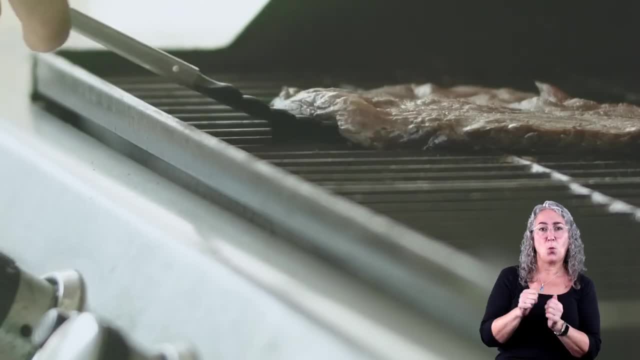 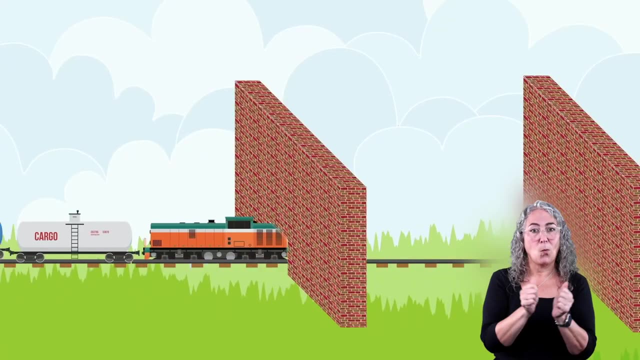 If you've ever seen your, If you've ever seen your parents cooking barbecue on a gas grill, the gas they're using is propane. It kind of goes without saying. but certain matter is easier to go through than other matter. You can swim in a liquid more easily than in a solid.